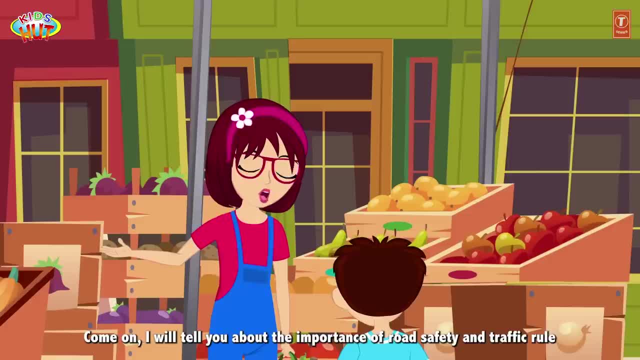 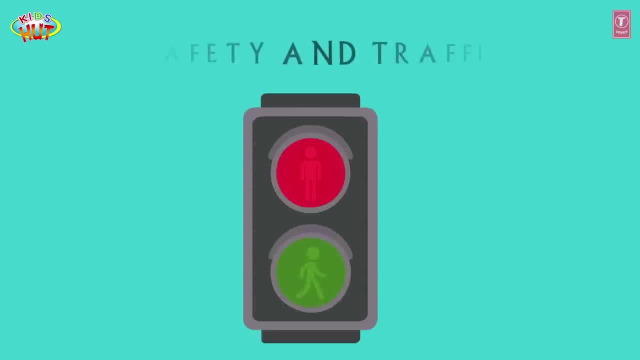 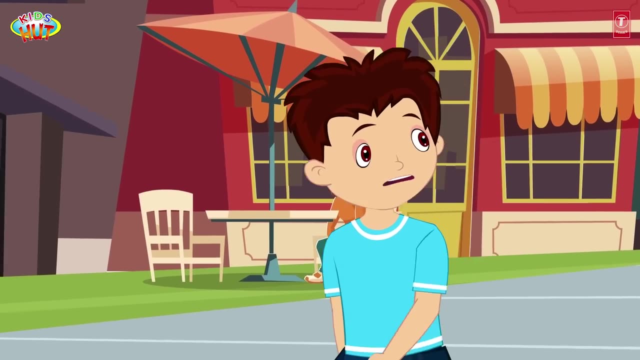 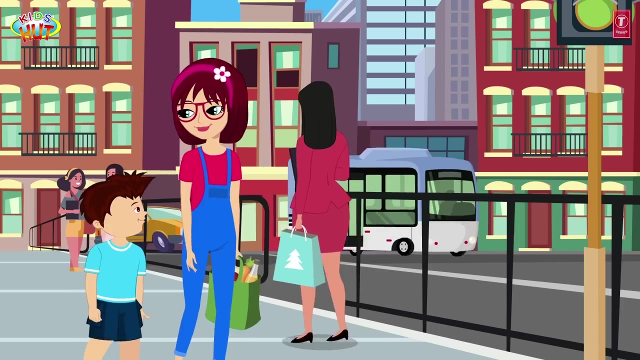 Come on, I will tell you about the importance of road safety and traffic rules. Please tell me, Tia. I saw the traffic lights while crossing, But I couldn't understand what the colours mean Very well. So here is the traffic light and this is the zebra crossing. 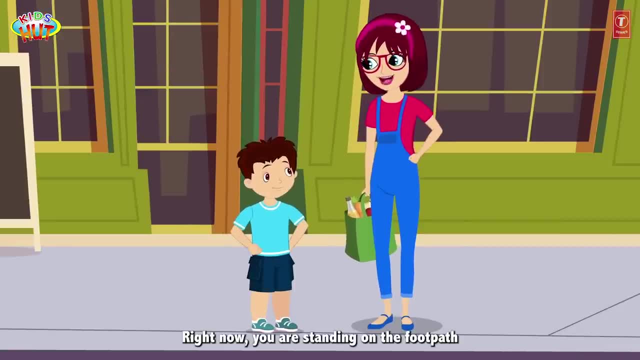 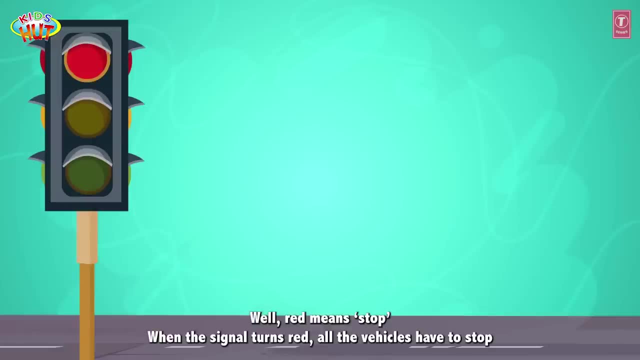 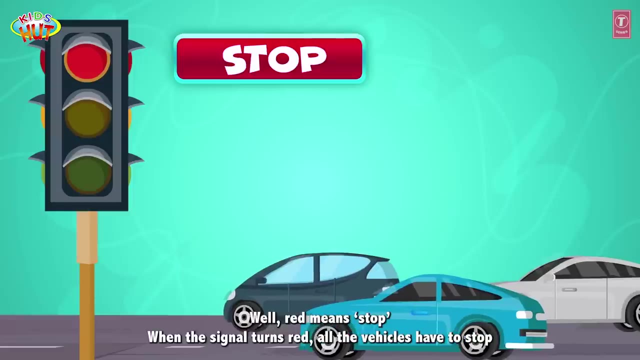 Right now you are standing on the footpath, I see. And what do these colours on the traffic signal mean? Well, red means stop. When the signal turns red, all the vehicles have to stop. The green light means stop. The yellow light means go. 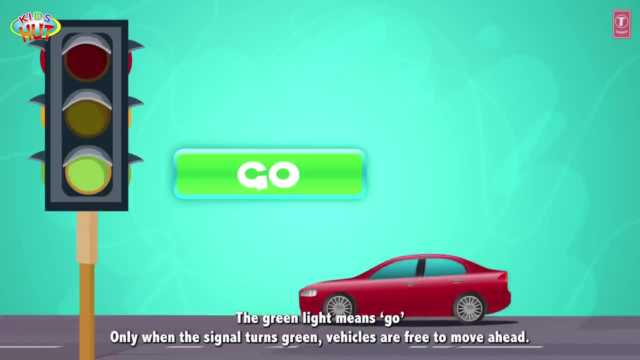 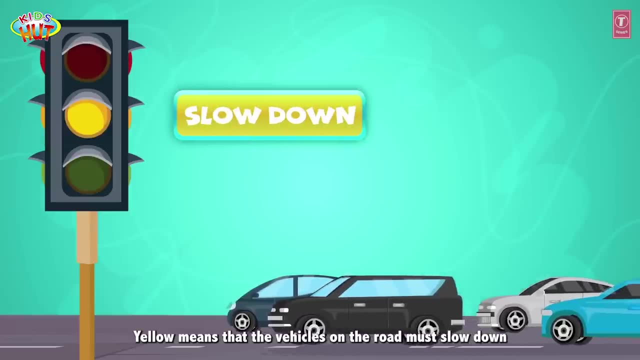 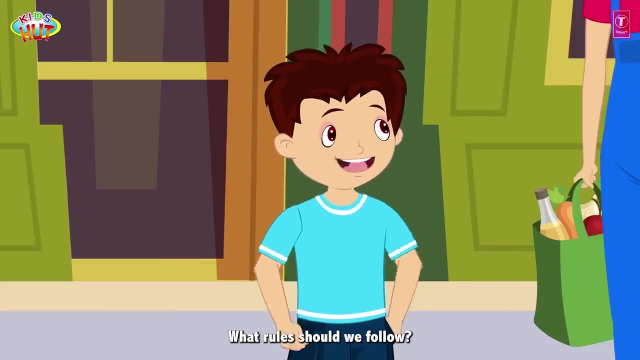 Only when the signal turns green, vehicles are free to move ahead. Yellow means that the vehicles on the road must slow down. These were the traffic rules for the vehicles, But what about us, Tia? What rules should we follow? Look there. 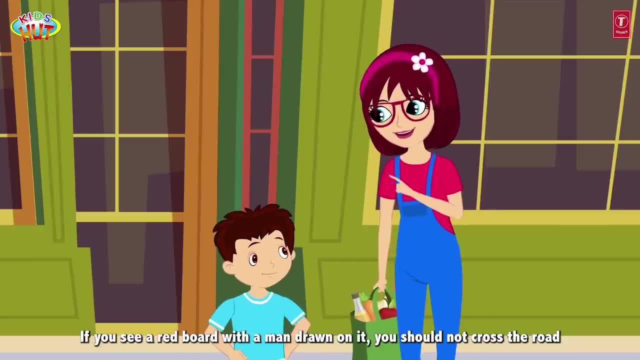 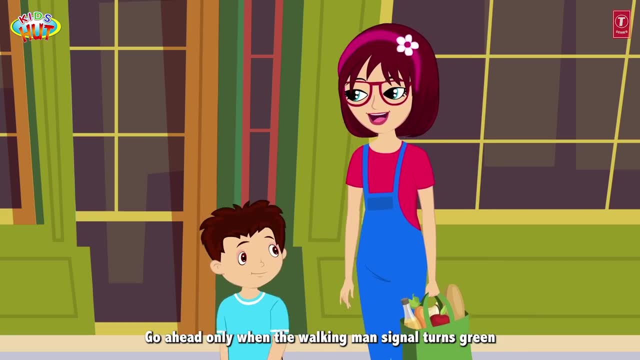 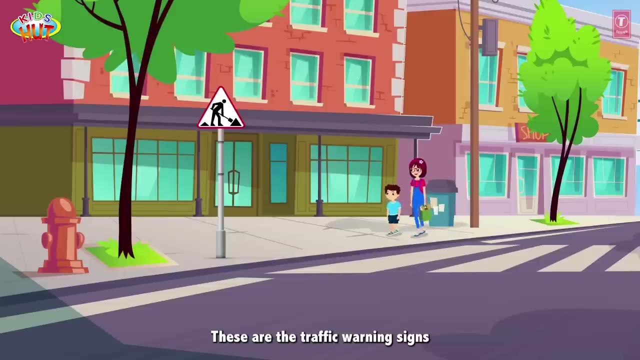 These signals are for the pedestrians. If you see a red board with a man drawn on it, you should not cross the road. Go ahead only when the walking man's signal turns green. Look, Tofu, these are the traffic warning signs. 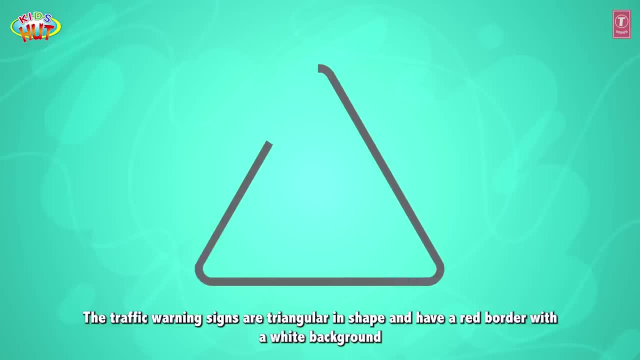 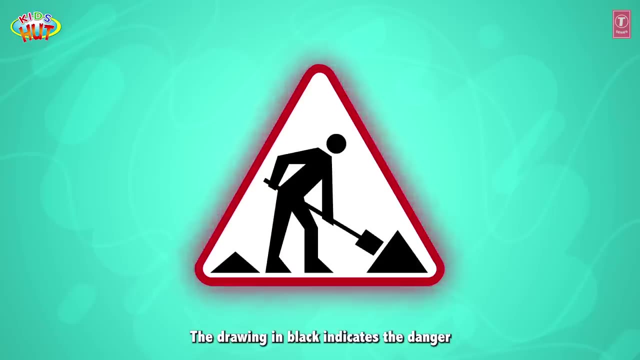 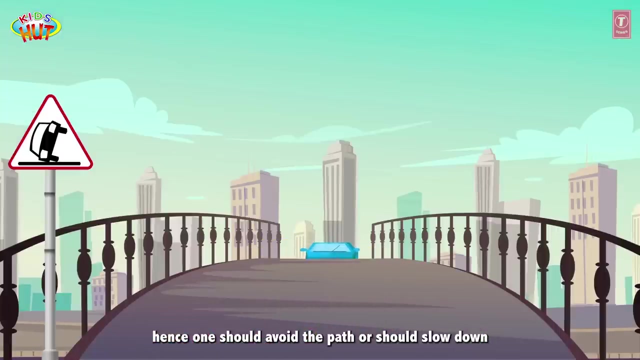 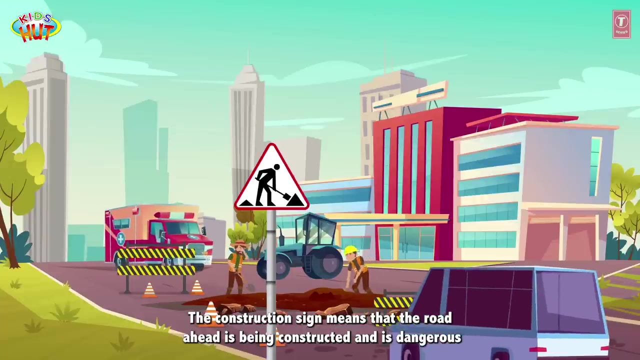 The traffic warning signs are triangular in shape and have a red border with a white background. The drawing in black indicates the danger. The slippery sign means that the road ahead is slippery, Hence the pedestrian should avoid the path or should slow down. The construction sign means that the road ahead is being constructed and is dangerous. 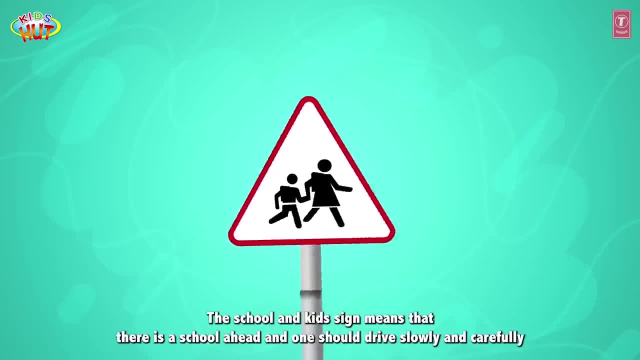 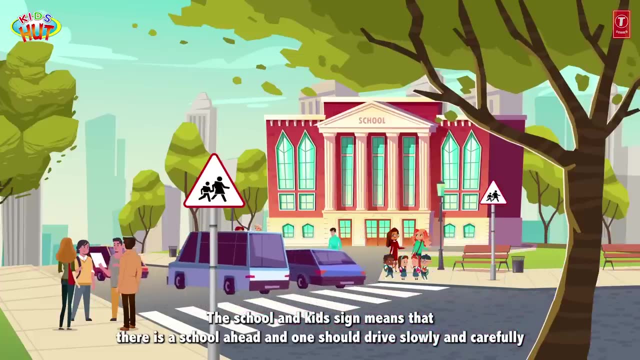 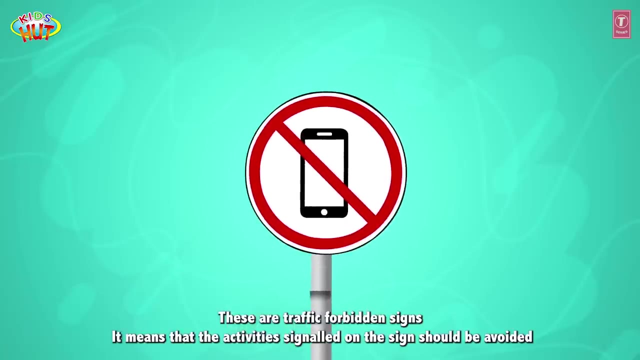 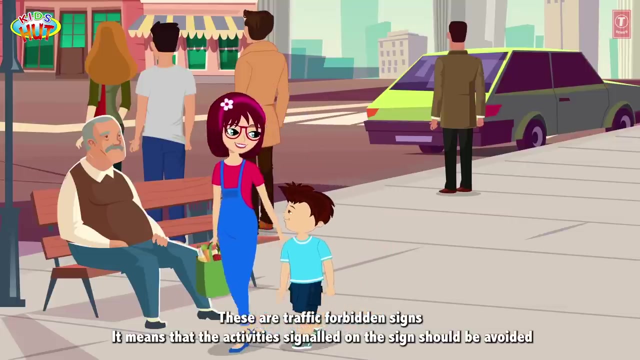 One should not go ahead. The school and kids sign means that there is a school ahead and one should drive slowly and carefully. Oh, I see. And what are those signs? These are traffic forbidden signs. It means that the activity signalled on the signs should be avoided. 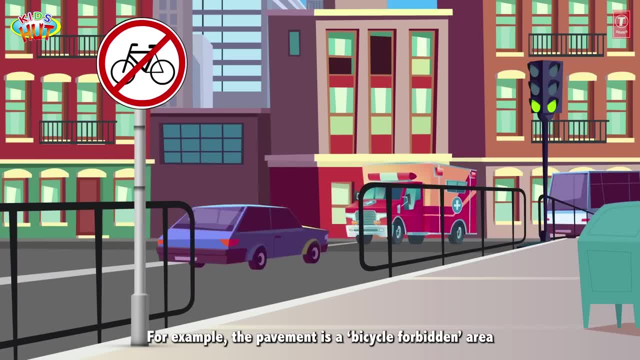 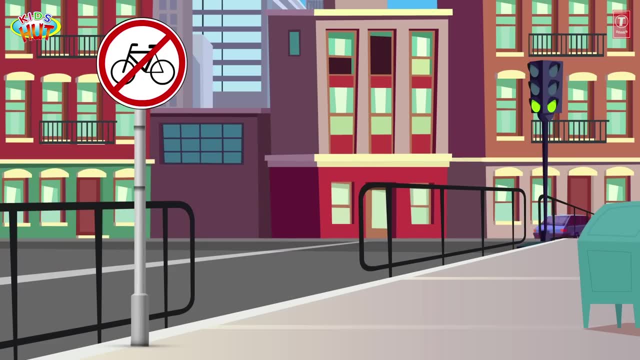 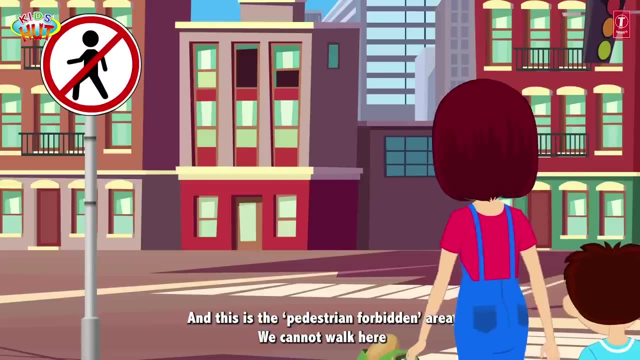 For example, the pavement is a bicycle forbidden area. You must not ride your bicycle here. This is for pedestrians only And there is a no entry area. You are restricted from entering this place And this is a pedestrian forbidden area. We cannot walk here. 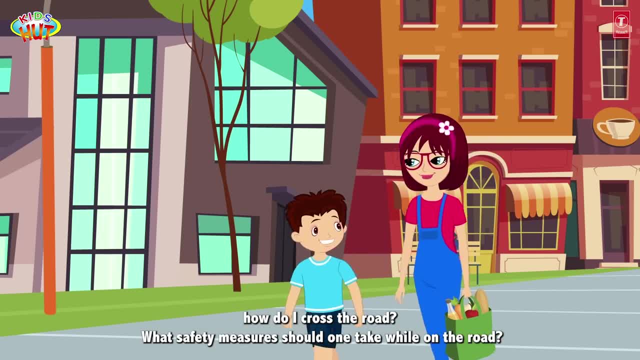 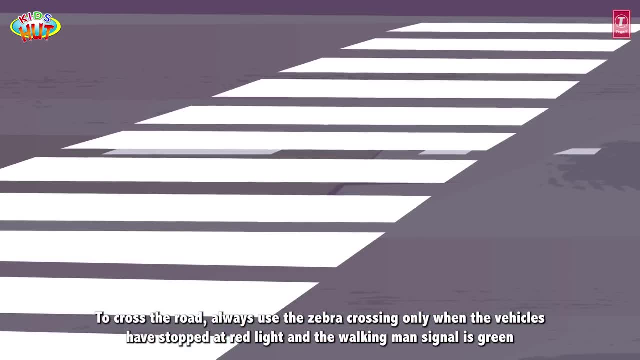 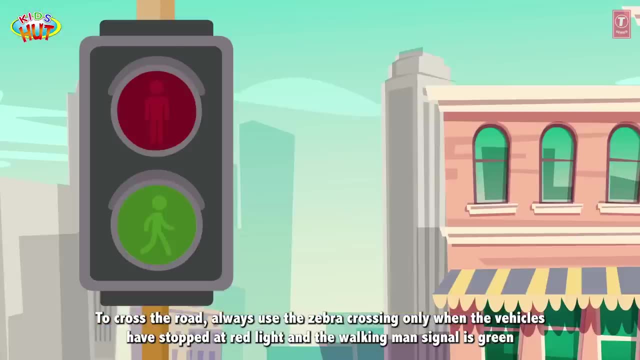 Okay, But Tia, how do I cross the road? What safety measures should one take while on the road? To cross the road? always use the zebra crossing only when the vehicles have stopped at the red light and the walking man signal is green. 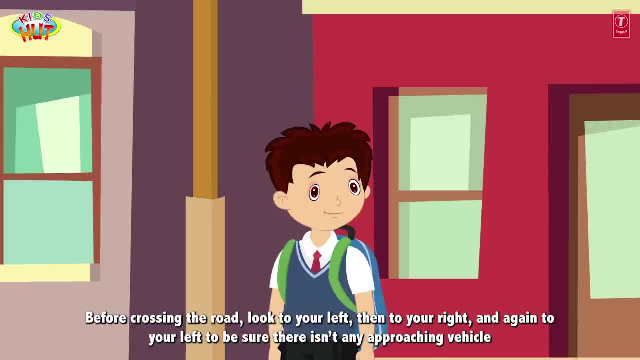 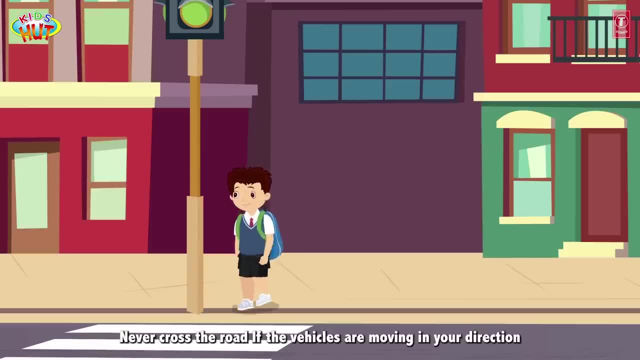 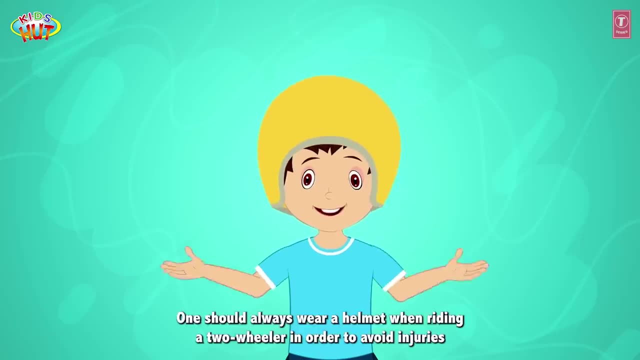 Before crossing the road, look to your left, then to your right and again to your left to be sure there isn't any approaching vehicle. Never cross the road if the vehicles are moving in your direction. One should always wear a helmet when riding a two-wheeler. 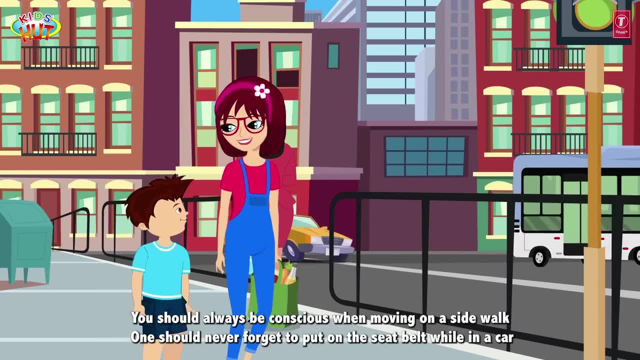 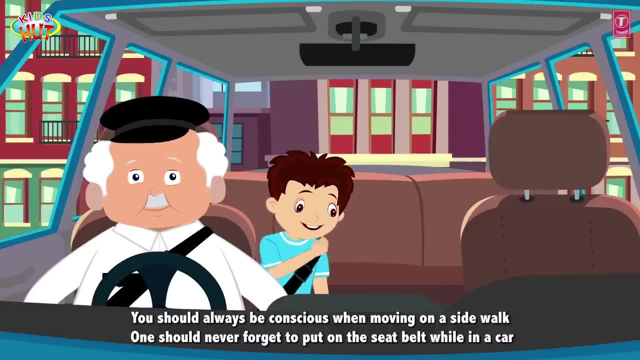 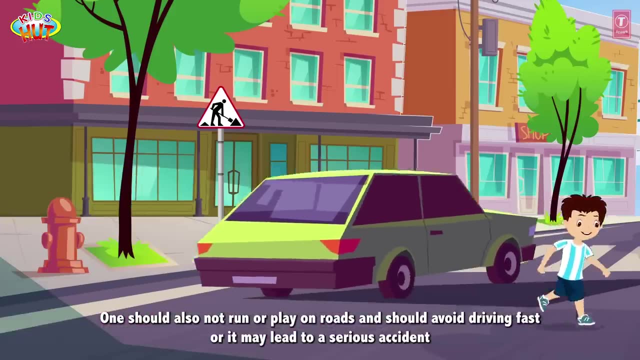 in order to avoid injuries, You should always be conscious. when moving on a sidewalk, One should never forget to put on the seat belt, while in a car, It protects us from harmful movements. One should also not run or play on roads and should avoid driving fast. 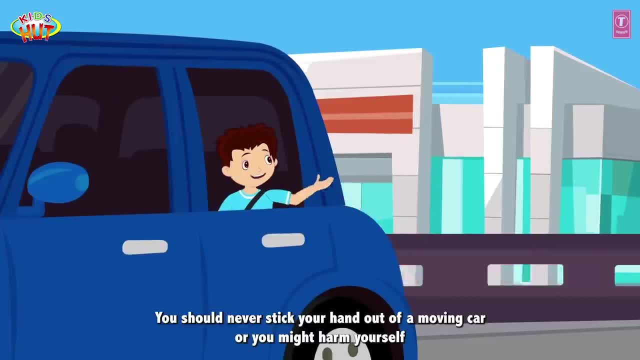 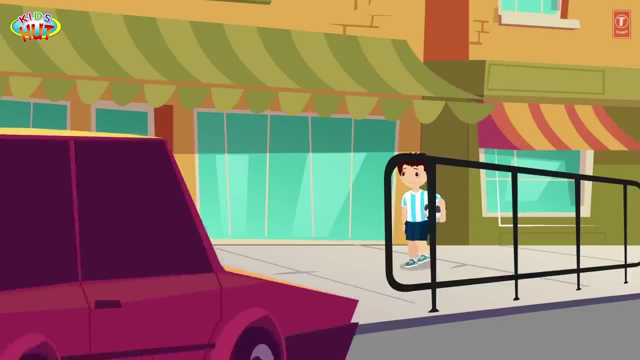 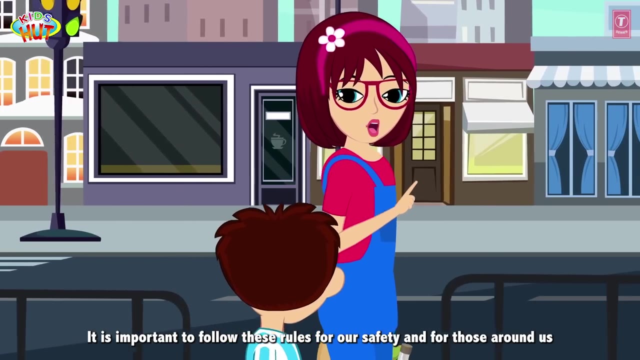 or it may lead to a serious accident. You should never stick your hand out of a moving car or you might harm yourself. Always use the footpath to walk. It is important to follow these rules for our safety and for those around us. Thank you, Tia, for sharing such an important topic with me. 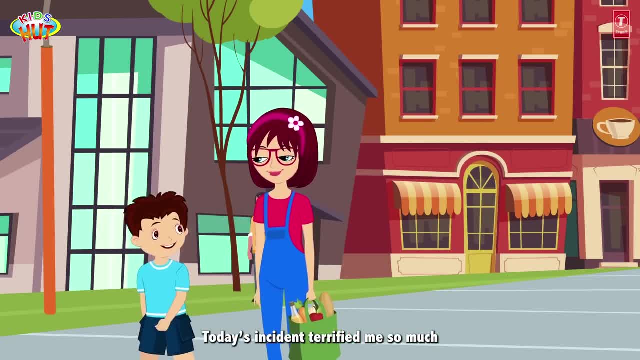 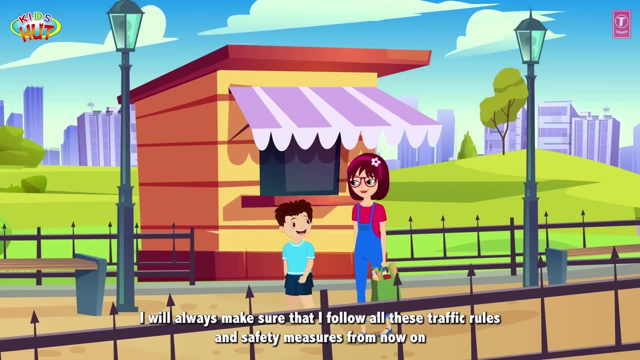 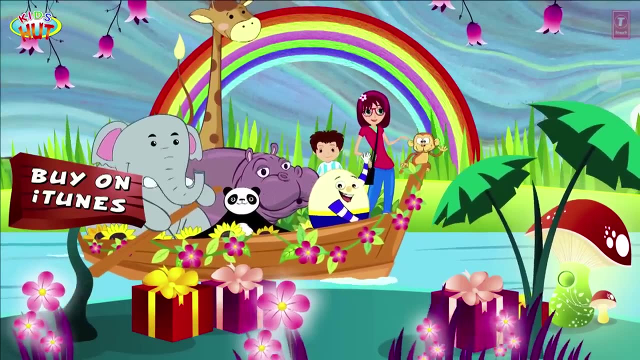 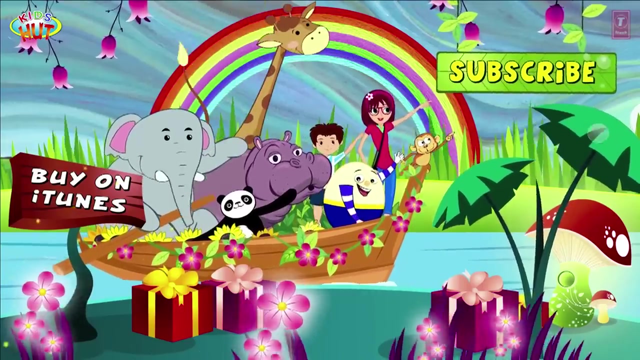 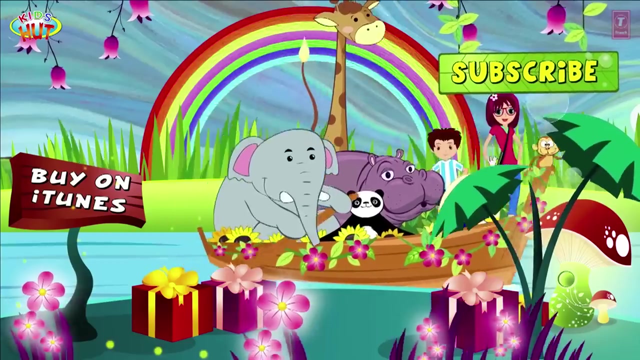 Today's incident terrified me so much. I will always make sure that I follow all these traffic rules and safety measures from now on. Thank you for watching. I hope you enjoyed the video. If you have any questions or comments, please let me know.